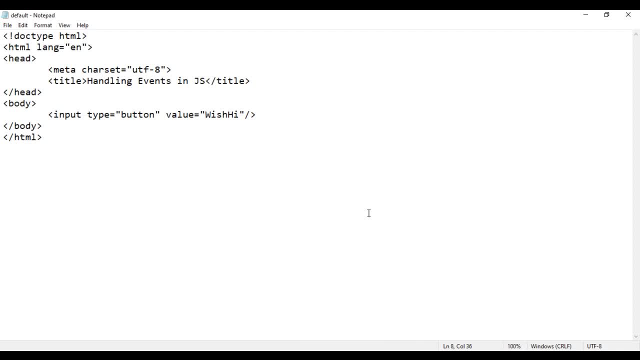 Either inline JavaScript or embedded JavaScript or external JavaScript. In inline JavaScript, what we do Here? we add an event OnClick. OnClick is a mouse event, guys. It is triggered when we click on that button, guys. There are many mouse events we have. 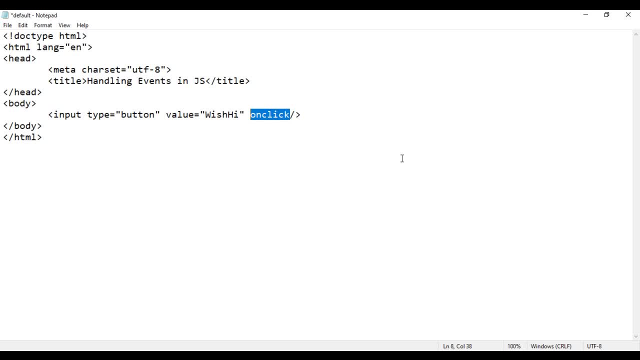 OnClick, OnDbClick. OnDbClick means on double click, OnMouseOver, OnMouseOut, etc. We have keyboard events like OnKeyDown, OnKeyUp. We have browser events, We have form events, We have image events. We have so many events, guys. 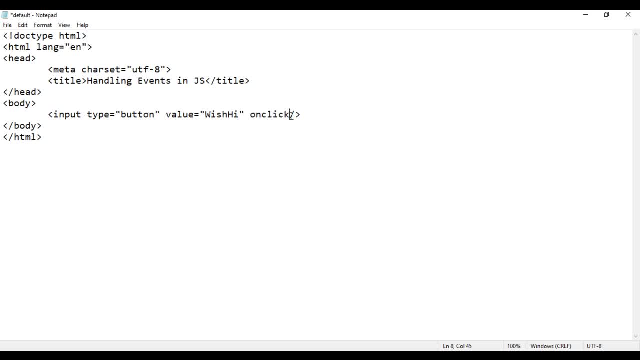 Here I am taking help of OnClick event, OnClick of this button. what should happen? Here? we write the JavaScript code directly inside the HTML tag. That's reason it is called as inline JavaScript. guys, Here I say alert, I am calling the alert function, which is a JavaScript function. 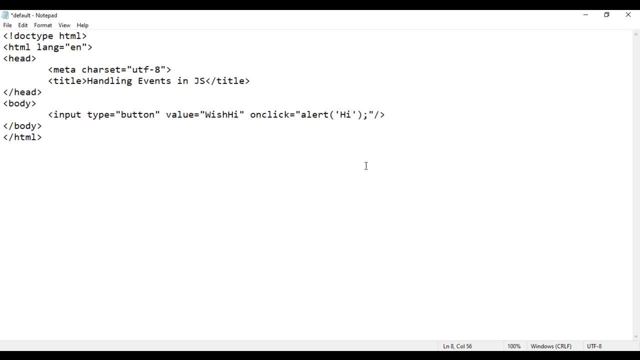 Inside single quotations I put the text hi. OnClick alert function should be executed. guys, If I save this, go to browser and reload. Now what happens? if I click on wish hi, We get the alert box saying hi, guys. If I click on this, we get an alert box saying hi. 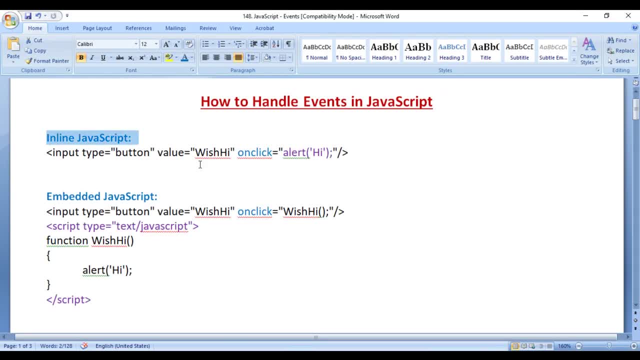 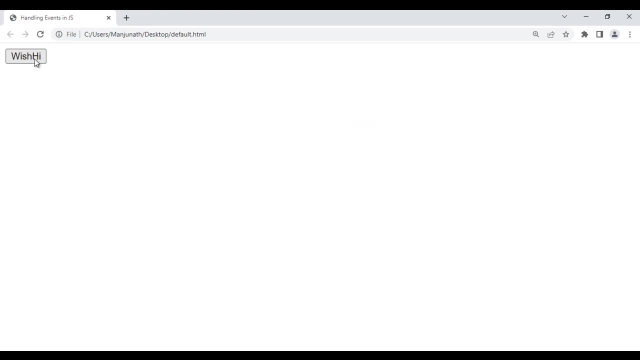 So this is called inline JavaScript. In inline JavaScript we write the JavaScript code directly in the HTML tag. Now I go back and remove this event, I save it, Go to browser and reload. If I click on this, nothing happens. We don't get the alert box because we have removed the event and the code. 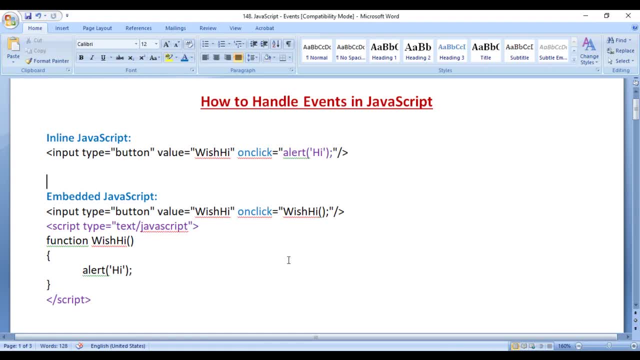 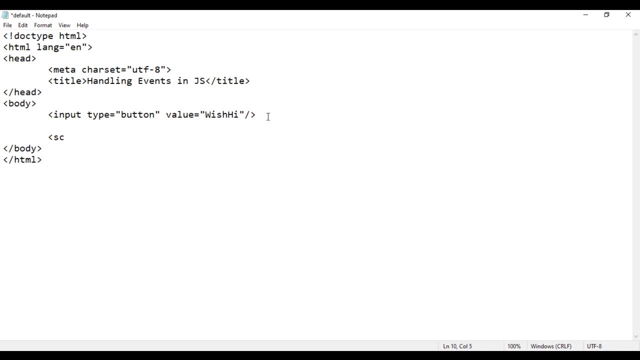 Let's understand how do we get that alert box saying hi using embedded JavaScript? What we do is we write here opening script tag and closing script tag And then I say here type is hi. Let's say here: type is equal to text or JavaScript. 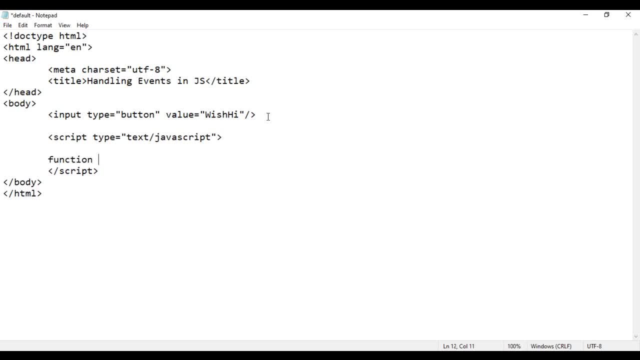 Inside this I am going to say function: wish hi bracket bracket. opening flower bracket. closing flower bracket. Inside the wish hi function, I call the alert function with the text hi guys. This function should be executed when we click on this button. For that again, I use the event onClick. 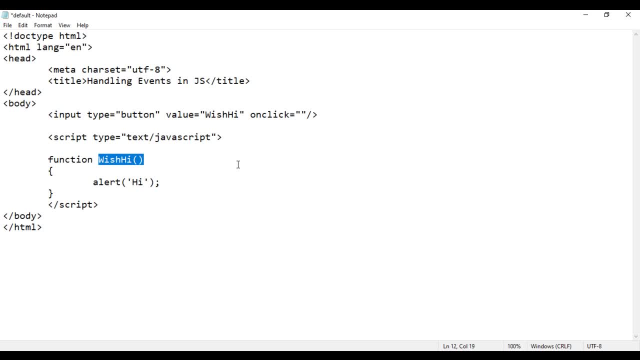 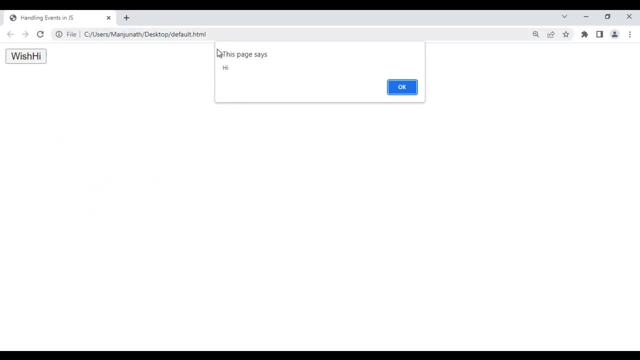 In double quotation. In double quotations I am going to say wish hi. Now I am telling: when I click on this button, wish hi function from JavaScript should be executed. If I save this, go to browser and reload, If I click on wish hi button, we get the alert box saying hi. 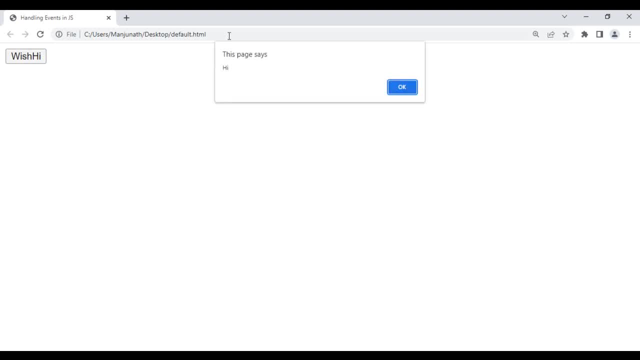 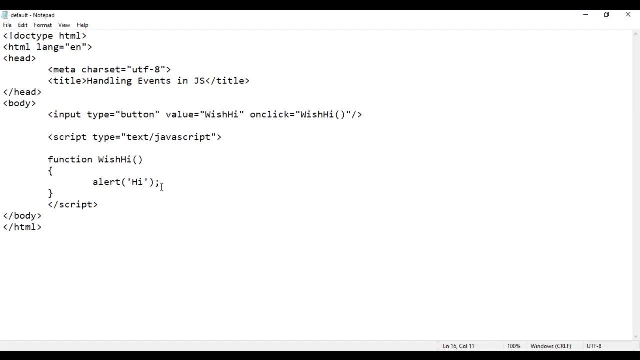 I say OK. I click again on wish hi, We get the alert box saying hi. If I click on this, we get the alert box saying hi. This is called embedded JavaScript, where we are creating a function inside the script tag And then we are executing this function on the event trigger. 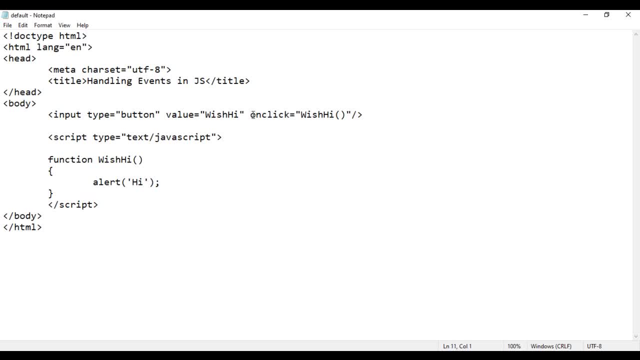 Right OnClick is the event guys. When the event is triggered, a function that we are calling here is called event handler. A function which handles the event is called event handler. guys. Now we have seen how we can display alert, How we can display alert hi, using inline JavaScript as well as embedded JavaScript. 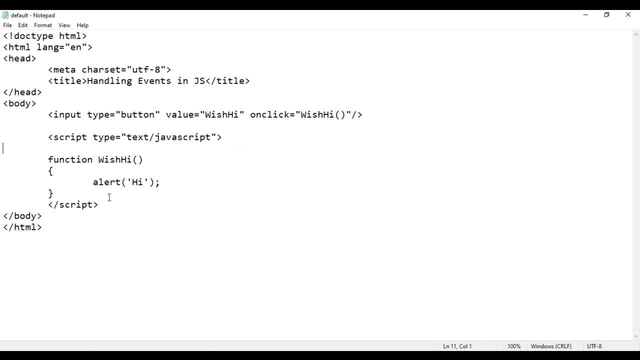 Let's do the same thing with the help of external JavaScript. I am going to delete this code. I remove this event, I save it, Go to browser and reload. If I click on this, nothing is happening. You can see that. 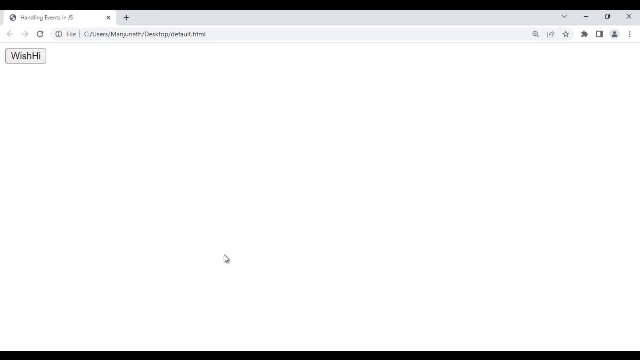 I am clicking, I am not getting the alert box, because we removed the code For external JavaScript. what we do? We create one new JavaScript file, guys, I say here notepad. In this file I am going to create function saying wish hi. 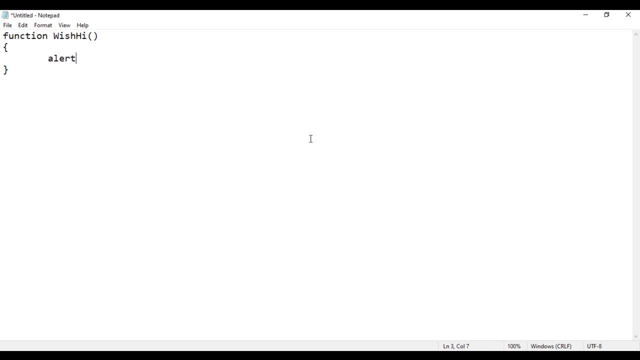 Bracket bracket- Opening, closing flower bracket. Inside that I call the alert function with the text hi. Now I am going to save it: File Save. as I save the file at the desktop with the name scriptsjs- Both sides, I put double quotations and save. 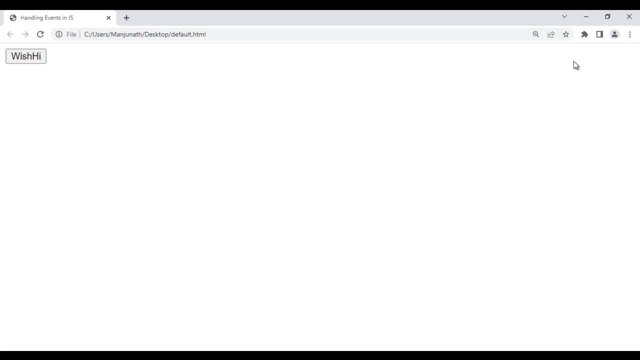 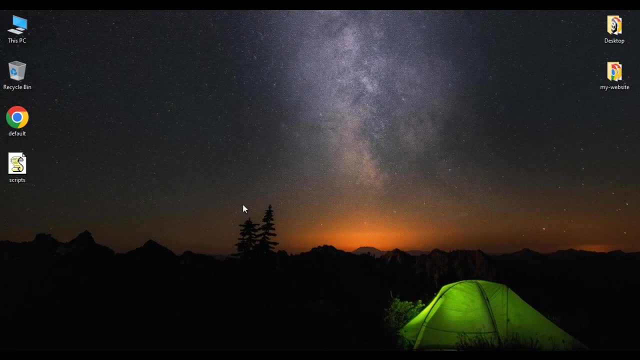 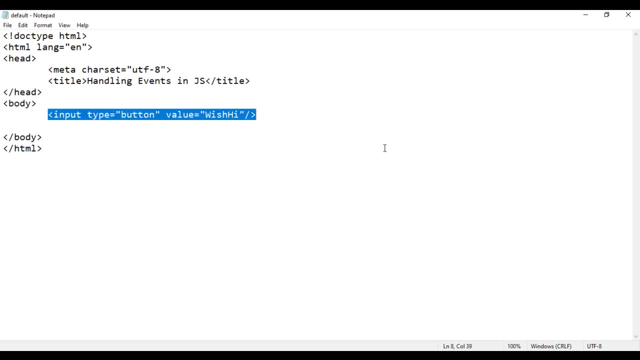 So I have an external JavaScript file Right. You can see, at the desktop we have a JavaScript file called scripts. In this script file we have wish hi function, which I want to execute When I click on this button. How do we do that? 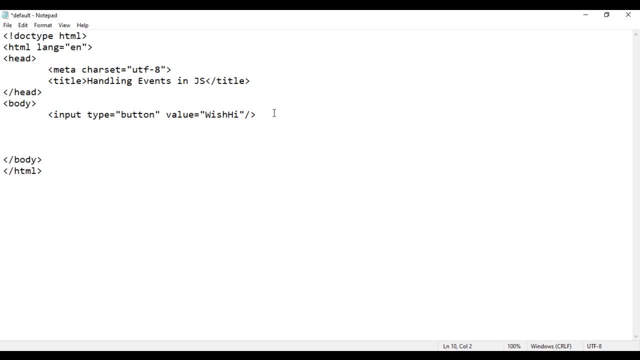 First we add that JavaScript file to our HTML page, guys, Using the script tag. I say here: opening script tag and closing script tag. And then I tell: use this source file called scriptsjs. And then I say here: type equal to text or JavaScript. 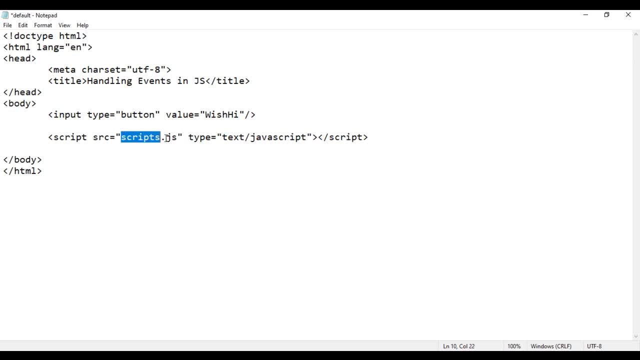 So this code adds this file to our HTML document. It adds that complete code from this file to our HTML document. guys, Now I say here on click: When I click on this button, You should call wish hi function. Wish hi function from JavaScript. 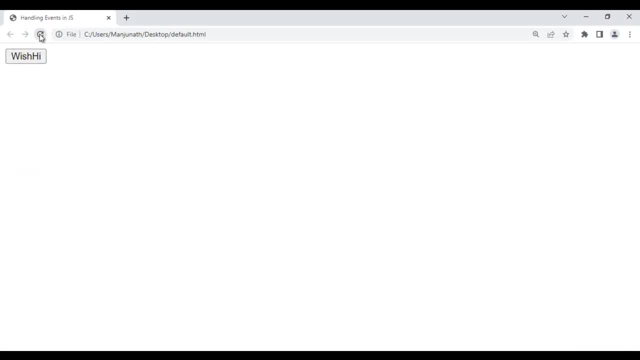 If I save this, Go to browser. Go to browser and reload. If I click on the wish hi button, We get the alert box saying hi. If I click on this Again, we get the alert box saying hi. So like this: 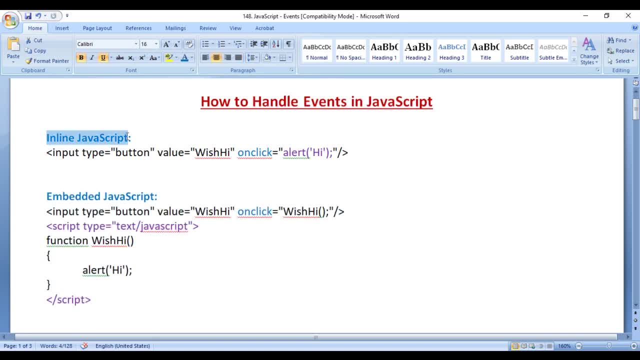 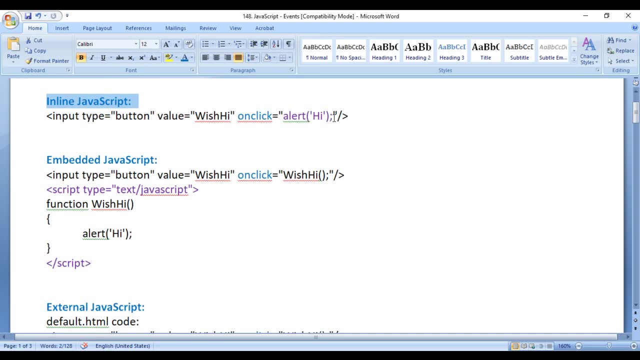 We can handle events in JavaScript Using either inline JavaScript Or embedded JavaScript Or external JavaScript. In inline JavaScript, We add the JavaScript code directly in the HTML element, Whereas in embedded JavaScript We create a function Inside the script tag And then we execute that function. 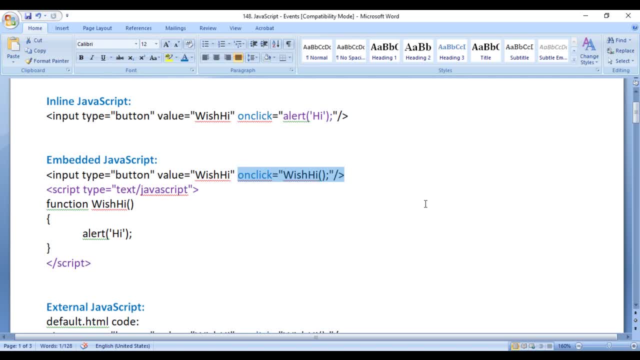 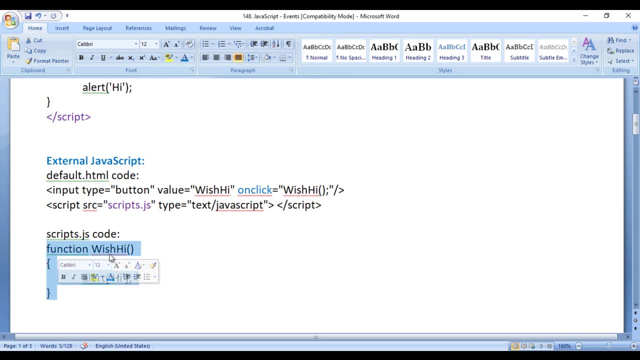 On a specific event trigger guys, Whereas in external JavaScript We create a separate JavaScript file With the function. We execute that function On the event trigger. Before that, we must and should include, We must and should add The script file to our HTML page. 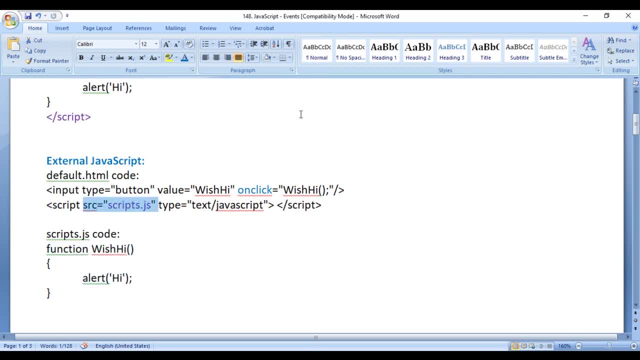 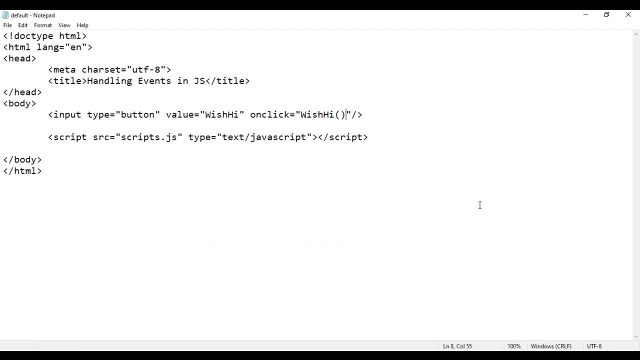 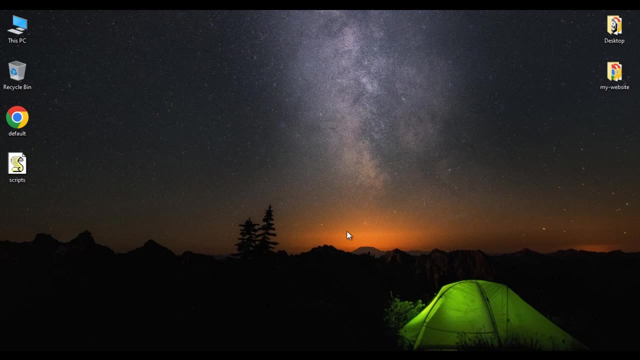 Using script src attribute. I hope you guys have Clearly understood. I suggest you people to Try whatever I explained Yourself And experiment. If you try and experiment You get more clear idea. guys, In the upcoming video tutorials We discuss more about. 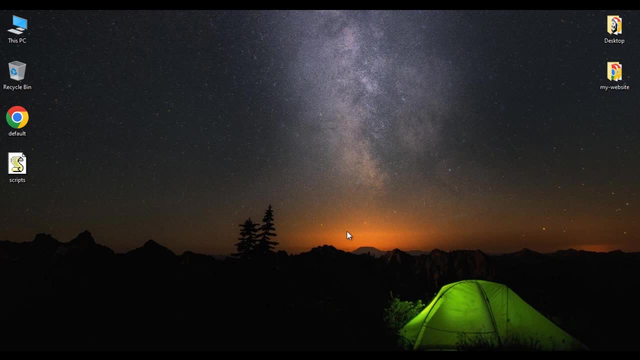 Handling events in JavaScript. If you like this video, Hit the like button And share with your friends So that everyone will get benefited. For more benefits And be up to date. Do not forget to subscribe To our YouTube channel. Keep learning. 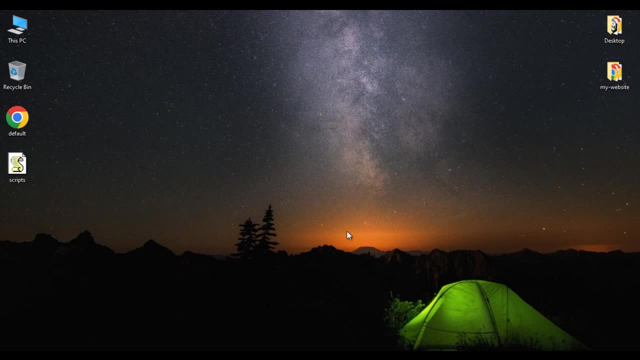 Keep coding, Keep sharing. Thank you guys, Thank you very much. See you In the next tutorial.